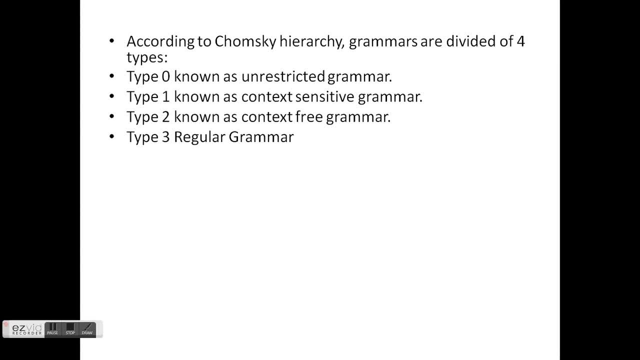 2, which is known as Context Free, and Type 3, which is known as Regular Grammar. So you should know which type of grammar is known as Context Sensitive or Context Free or Regular Grammar. Next, to recognize all these types of grammar, how to know which is Type 0, Type 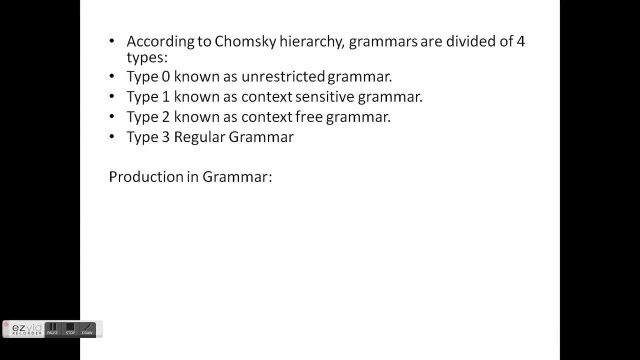 1 or Type 2.. We must know about production. So what is production in grammar? These are some examples of production. Now you can see there are some capital letters in this or some small letters. Capital letters are called non-terminal and small letters are called terminal. Now 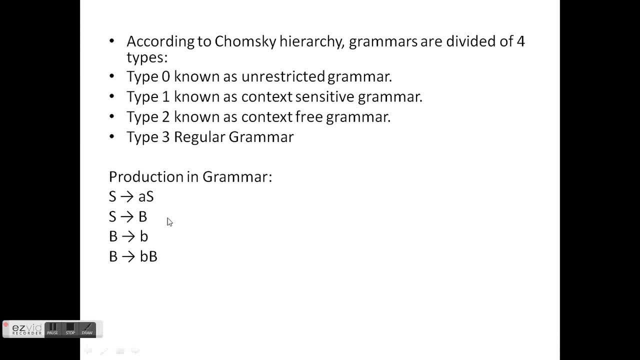 what is the difference between terminal and non-terminal? Non-terminal means some more substitutes can be done in place of this. For example, S drive B and B replaced by small B. again, What is terminal If I did B drive B and now I can't substitute any more in place of 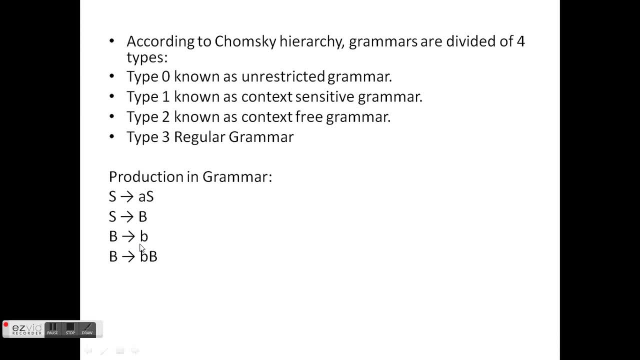 small B. So this is terminal. You must remember one thing: how to know which is terminal and non-terminal: Those which are written in capital letters, those are called non-terminals, and those which are in small letters, those are called terminals. So capital letters are. 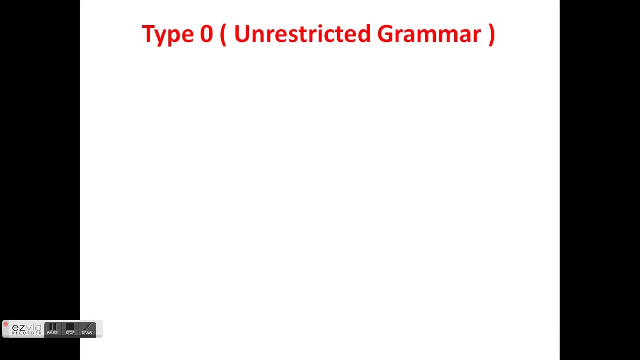 non-terminal and small letters are terminals. Next, type 0, which is called Unrestricted Grammar. These type of grammar include all formal grammar. This is recognized by Turing Machine. Do remember one thing: the question arises that which machine recognizes type 0 and which? 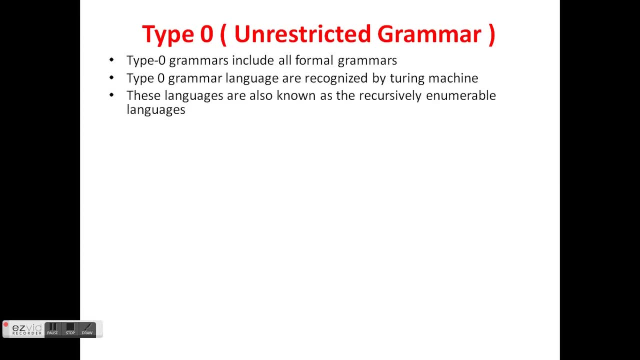 machine recognizes type 1.. So type 0 is recognized by Turing Machine. These are also called recursively enumerable languages. Now how to know which language is type 0? This is very simple: Type In type 0, in which the production is in the type of alpha drive beta. 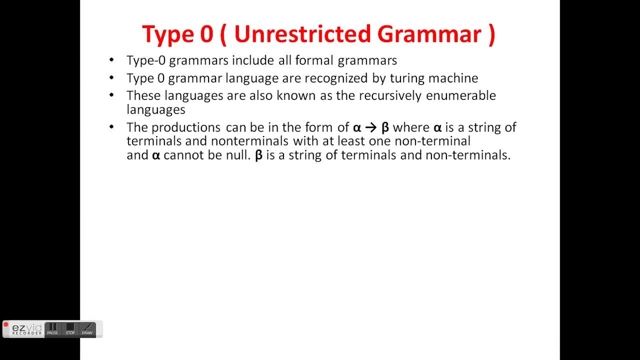 What is alpha String of terminal and non-terminal Means on the left side, which is alpha, Anything can come, Any terminal, any non-terminal can come. But at least one non-terminal should come on the alpha side And there is no restriction on the beta side. Anything can come. 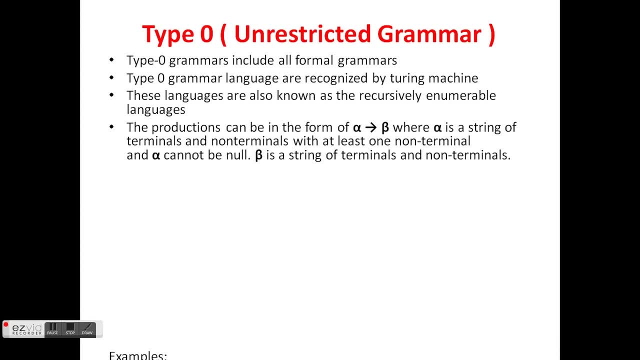 Whether the terminal comes, whether the non-terminal comes, Whether any combination comes. Let's see the examples. See the first example: A, C, A B. There is one on the left side, Any combination on the right side. Type 0. What is here? Type 0. 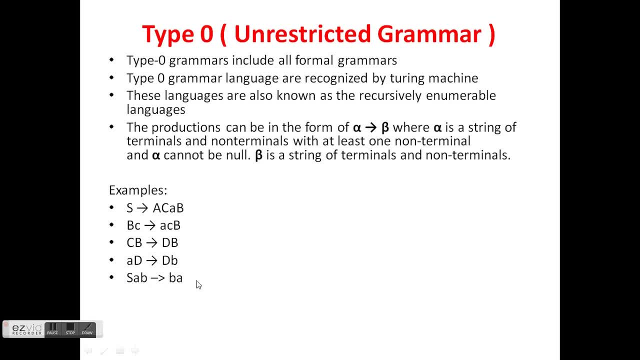 Type 0 In the fourth example too. What is this Type 0, What is this? in this too, Type 0 Means. at least one non-terminal should come. There is also a non-terminal in this. In the first one too, There is also a non-terminal in this. 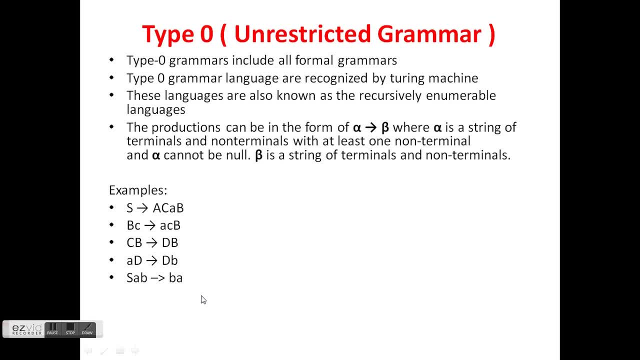 There is also in this. There is also in this. So what is this? Type 0? There is no restriction, See alpha. Alpha is also greater than beta in this case. In the case of alpha, The length here is 3. What is here? Beta is 2. So what happened? 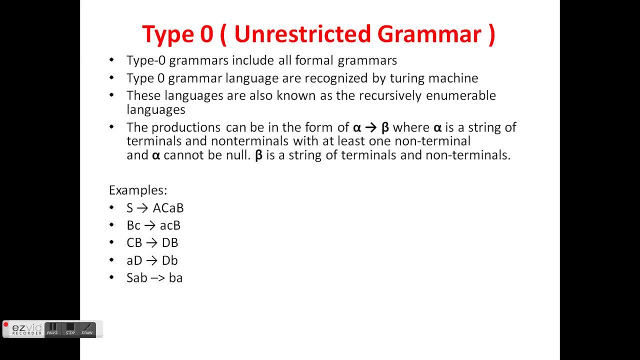 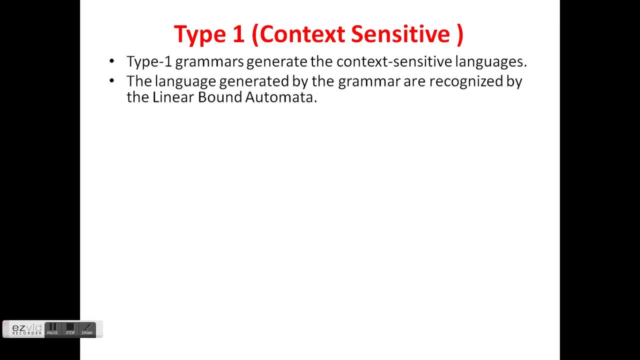 Type 0 Means there is no restriction In type 1. We will see that the restriction came. How did it come? Let's see that Next. Type 1: Context sensitive. These are recognized by linear bound automata. Remember, Type 0 is recognized by Turing machine And this is recognized by linear bound automata. 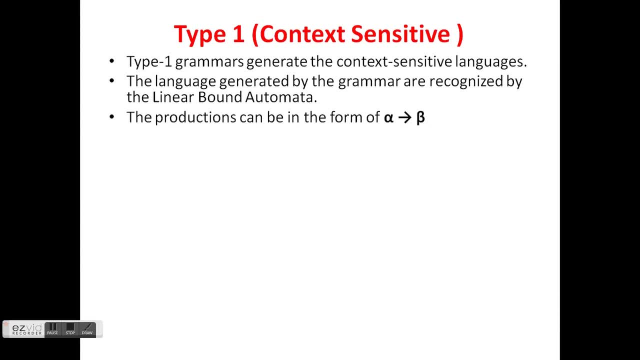 Type 1 Production. again, Form alpha derives beta. Only one restriction. There is only one restriction in this: The length of alpha must be less than or equal to the length of beta. Here you can see: The length of alpha is less than beta in every case, And again the alpha side can also come. 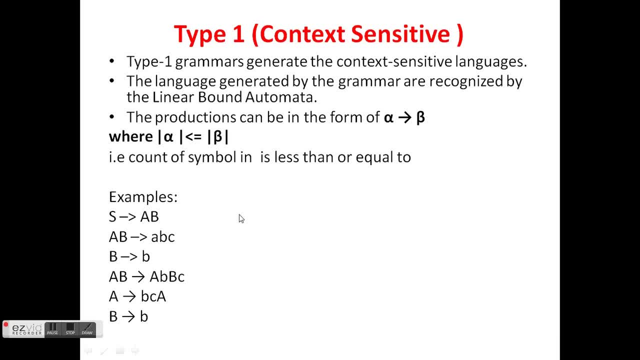 The beta side can also come. It is simple. What is the difference between type 0 and type 1? In type 0 The length of alpha can be greater than beta, But in this The length of alpha Will be less than beta, Where The length of alpha is equal to beta. 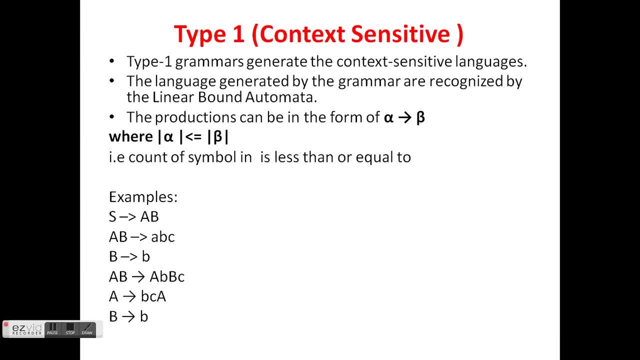 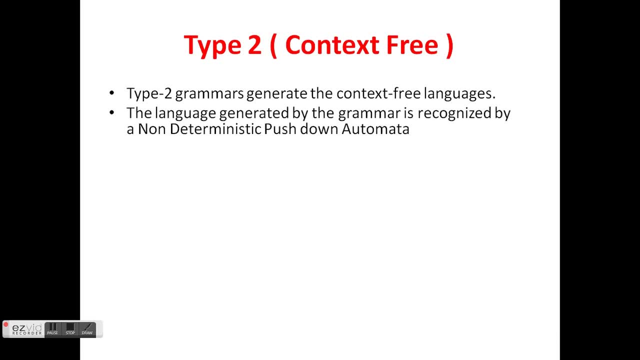 Next We will see type 2. Now What other restriction came in it. Let's see Type 2. We call it Context free. These are recognized by pushdown automata. Now Let's see What was in type 0. The length of alpha is anything. It is also greater than beta. 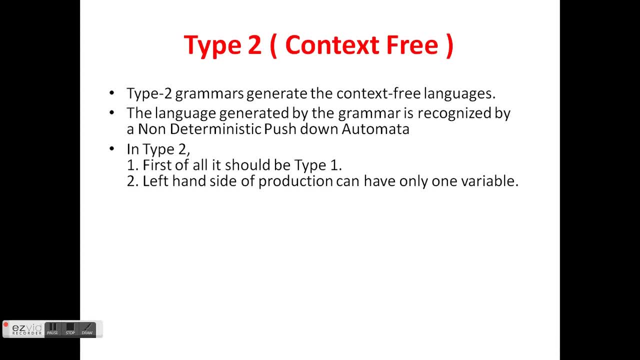 No problem. What is in type 1? The length of alpha Must be less than beta. But in this, What is the length of alpha? It should be one, But in this The length of alpha Must be one. So What is in type 2, The length of alpha? 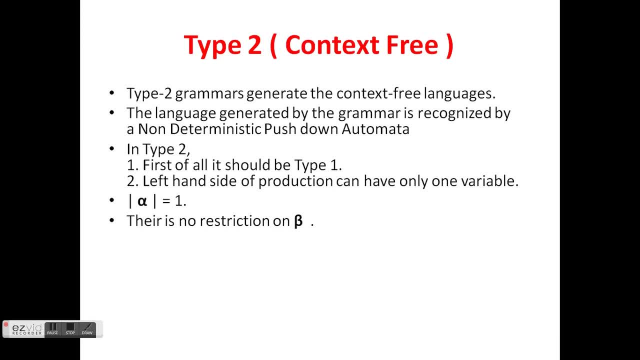 Must be one. So The length of alpha Equals to one And There is no restriction on beta. No, You can see Here, In all three examples, Alpha On the left side There is only one Variable. There is only one variable Which is Non-terminal: Anything can come. on the right side, 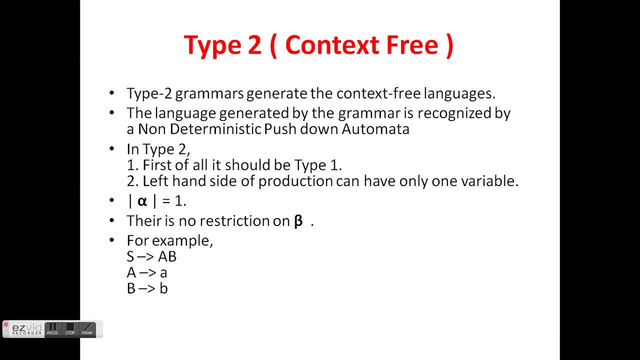 Means. There is no restriction on beta. There is no restriction on the right side, No. Next We see type 3, Which we call Regular grammar. Now what will happen in that? There will be a restriction on beta In this. What is in type alpha? There will be a restriction on beta. 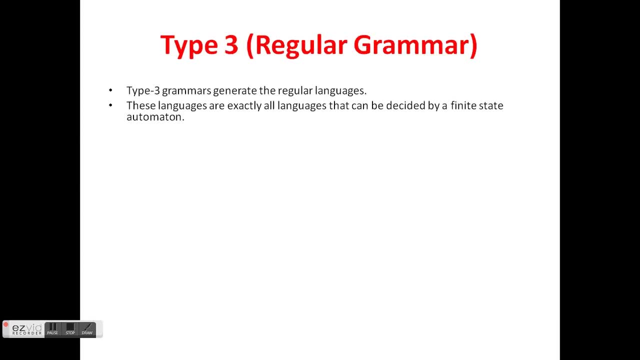 So Type 3, Regular grammar. These are recognized by Finite state automata. I repeat: Type 0: Turing machine. Type 1: Linear bound automata. Type 2: Pushdown automata. Type 3: Finite state automata. This is most restricted. What was type 0? 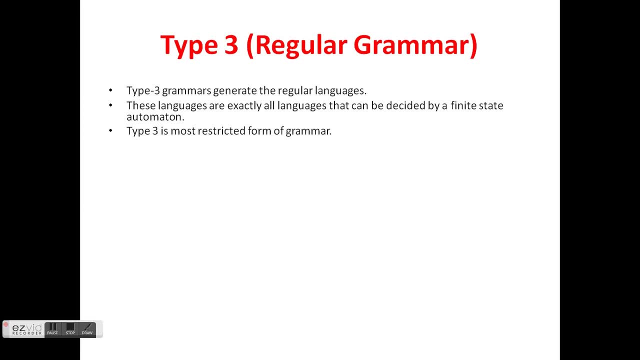 Unrestricted. Now, What is in this? On the left side, There is a single Non-terminal Which is Unrestricted. There should be a single Non-terminal. That is obvious, Because it is derived from type 2. Now, In type 2, There was only one on the left side. 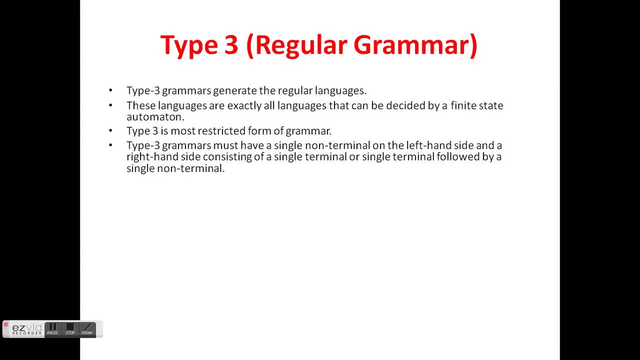 Alpha 1. But what is in this? On the right side, Where there will be a single terminal, Where After the single terminal Non-terminal, For example, See X drive A Single terminal, Where X drive A Y After the terminal Non-terminal. So what happened? Regular grammar, Nothing can come on the beta side. 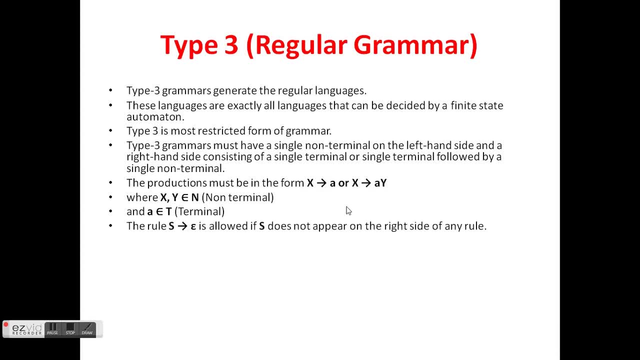 This is Whatever. This is In this. One more rule: Allowed X drive Null. There is also null production in this, In type 3. There is no other. This is not. You can see examples, As I said before, On the right side, Where there is a simple Non-terminal. 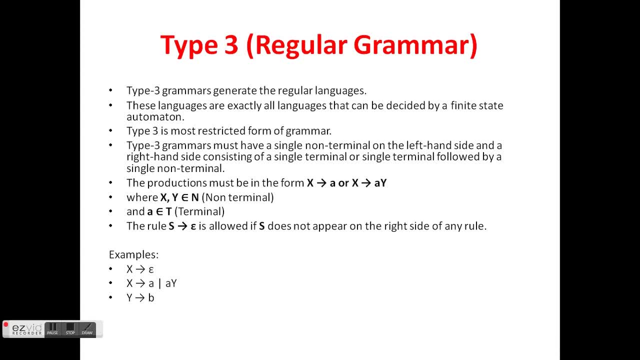 Sorry, Terminal Where If Non-terminal Does not come, Then it will After the terminal. I hope You have Enjoyed This video. If there is any doubt, In the comment section You can comment. You can watch the video And, yes, In this Three questions At least, You will come to CBSE. 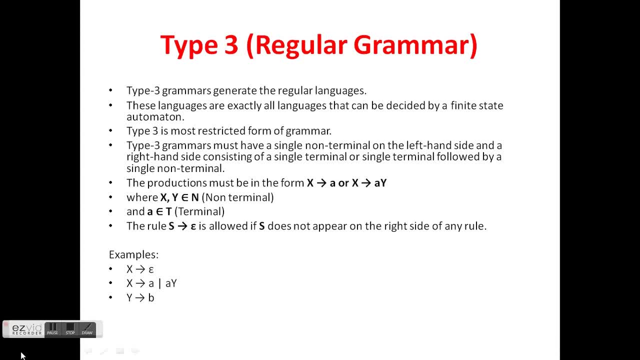 Net Will come To see. Thank you. You can subscribe to the channel.